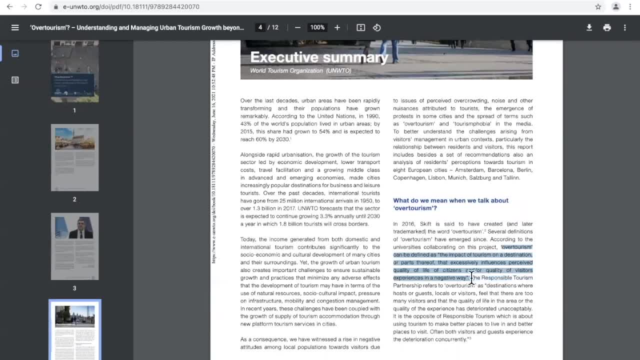 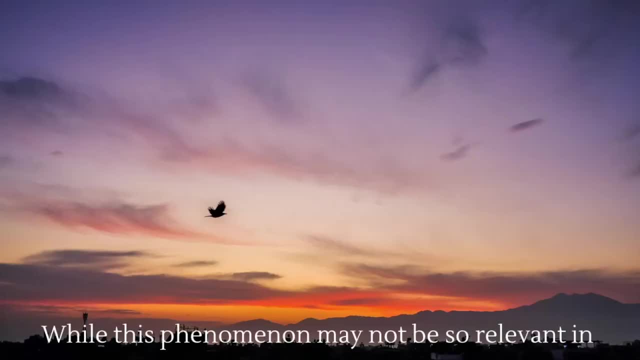 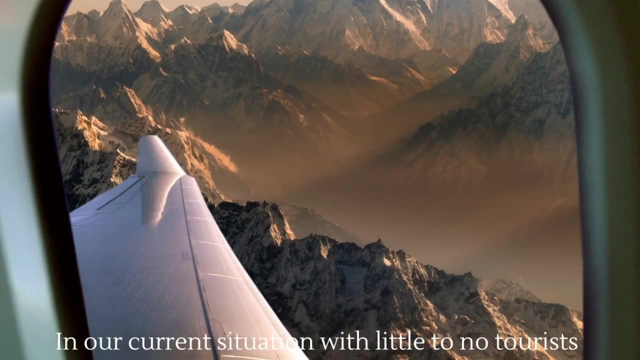 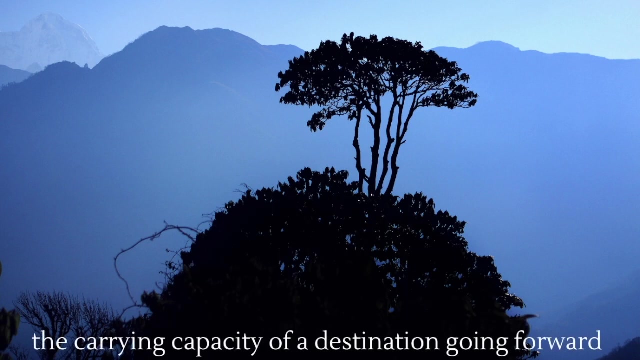 perceived quality of life of citizens and or quality of visitors' experiences in a negative way. While this phenomena may not be so relevant in our current situation with little to no tourists, it is crucial that we pay attention to the carrying capacity of a destination going forward. 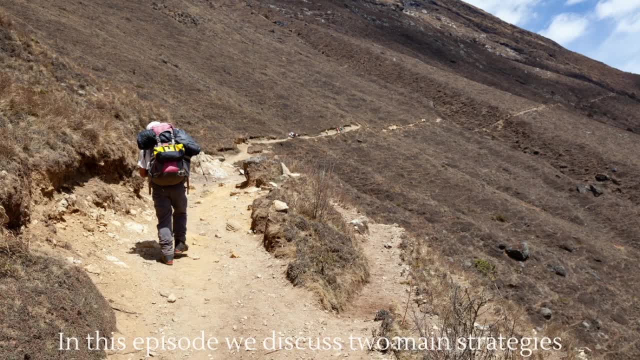 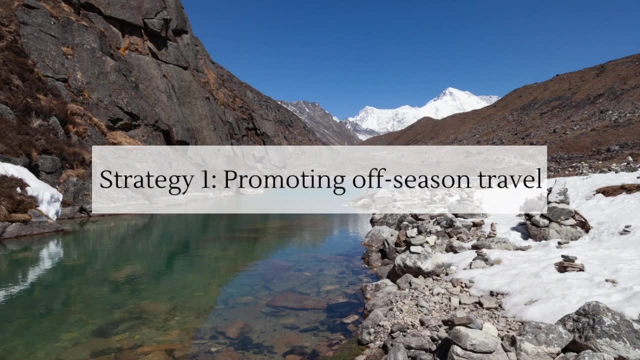 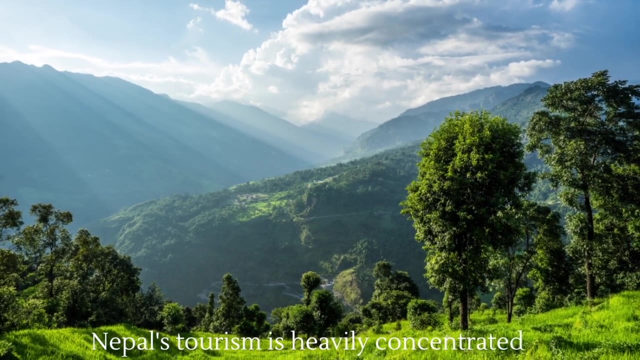 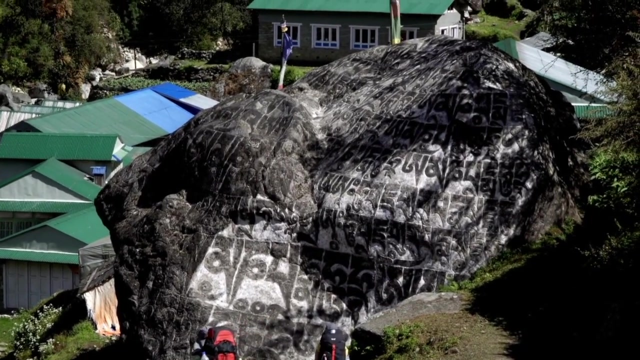 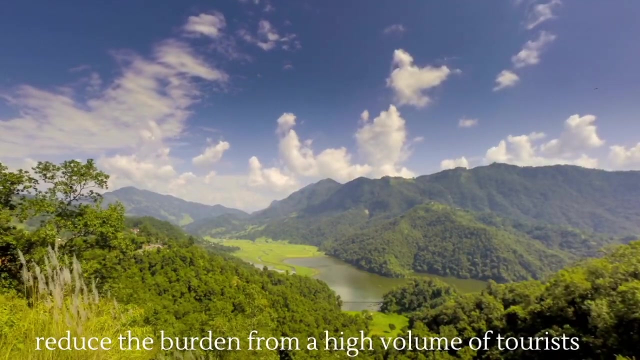 In this episode we discuss two main strategies to address overtourism. Nepal's tourism is heavily concentrated in the months of March to May and September to November. By promoting off-season travel, we can reduce the burden from a high volume of tourists in a given destination. TANOR NOR- FOUNDER OF TANOR TOURISM, IS A TOURISM CONCENTRATION IN THE MONTHS OF MARCH TO MAY AND SEPTEMBER TO NOVEMBER. TANOR NOR IS THE FIRST TOURISM CONCENTRATION IN THE MONTHS OF MARCH TO MAY AND SEPTEMBER TO. 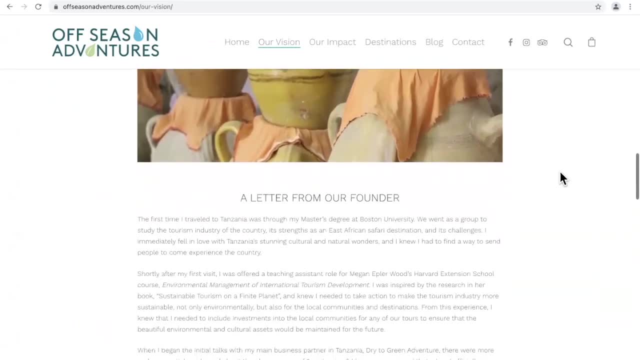 NOVEMBER. TANOR NOR IS THE FIRST TOURISM CONCENTRATION IN THE MONTHS OF MARCH TO MAY AND SEPTEMBER TO NOVEMBER. TANOR NOR'S RESPONSIBILITY OF OFF-SEASON ADVENTURES HAS MORE TO SAY ON THIS. 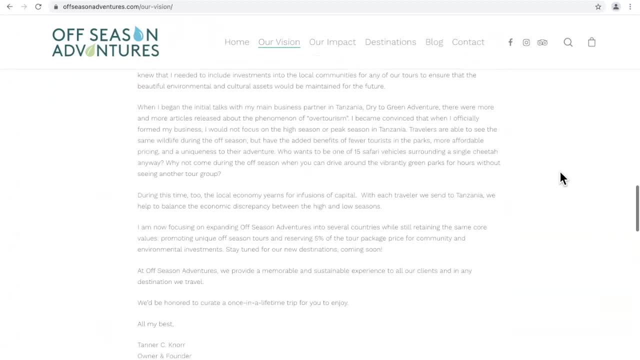 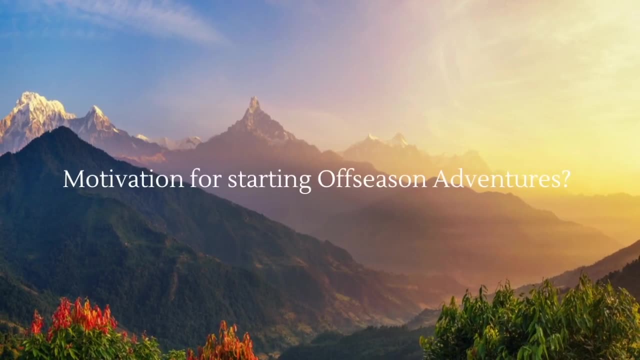 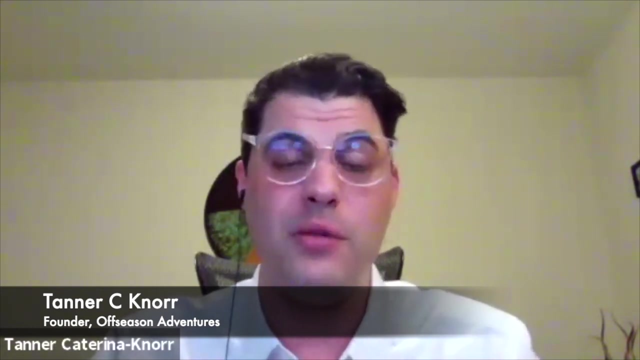 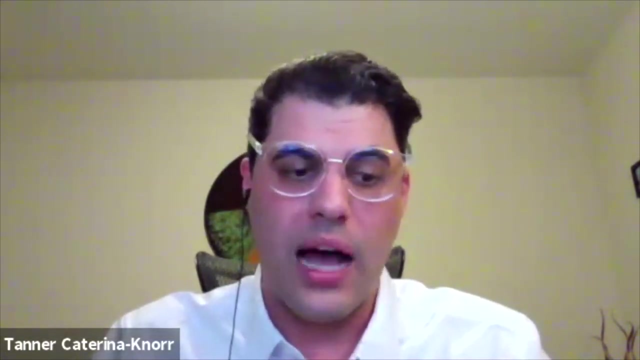 Off-season adventures began a few years ago, and our first destination was Tanzania, Eastern Africa. I went there for a class trip and when I was around, I could only fly a drone. It was a revolution. It was in my 봅 estamos. 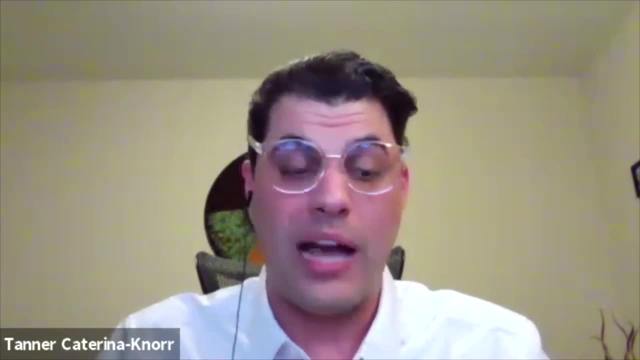 I was there. it was during the off-season and I looked around and I said, wow, there's so many wonderful things to see here in the off-season, and what I'm seeing here is not what's typically displayed on the tourism websites. We were having conversations with locals. The entire country was. 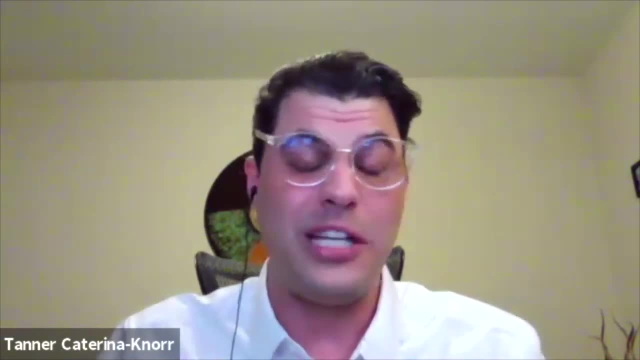 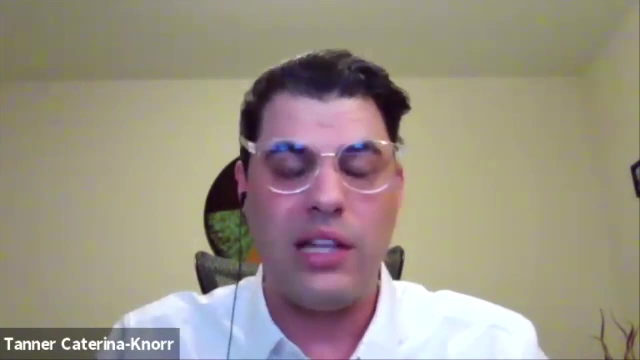 lush and green and there was virtually no one around. We would drive for hours in the national parks without seeing anyone and I thought, well, this would be a really great idea to bring to other countries, and I hadn't heard of a tour company focusing specifically on the off-season. 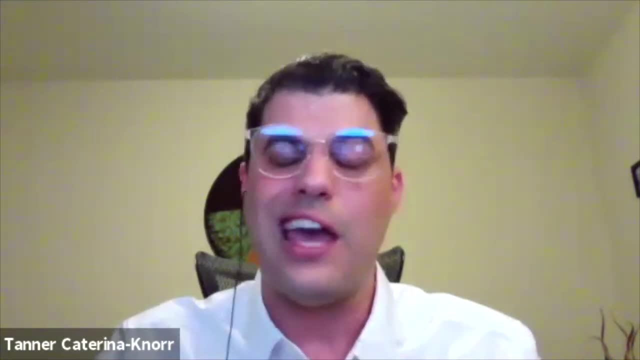 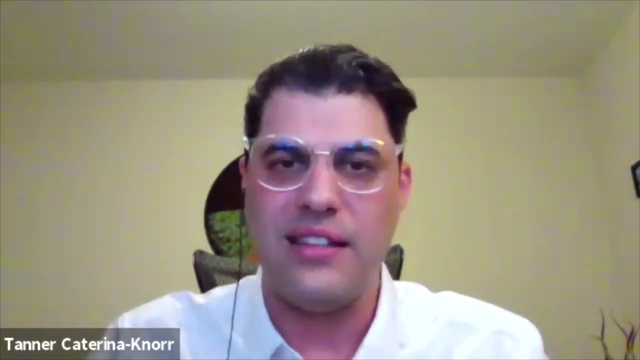 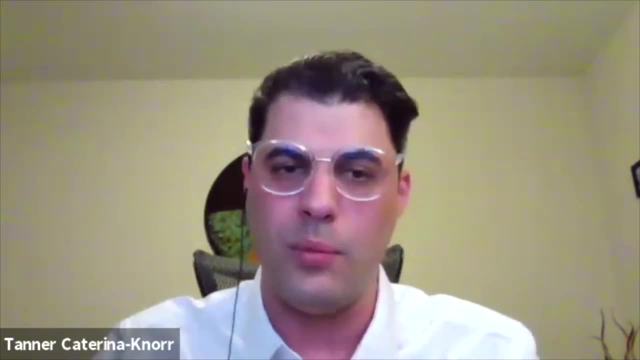 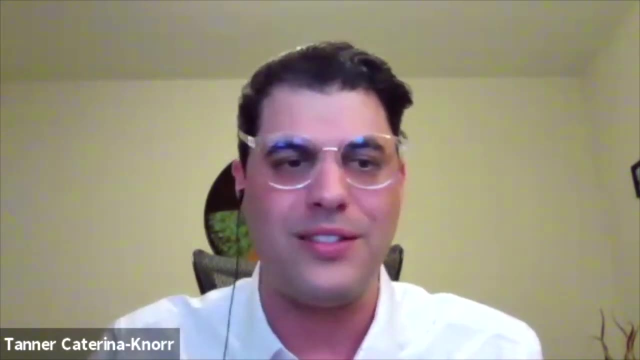 It's a personal connection between the traveler and the local people. You can have longer conversations without feeling like you're part of a conveyor belt of tourists- during the high season perhaps- and then being able to drive around the national parks and the trails without having a lot. 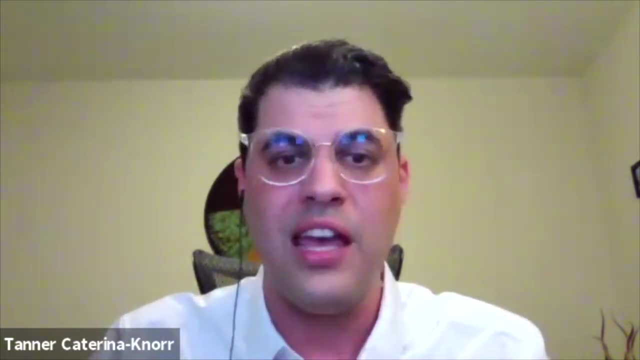 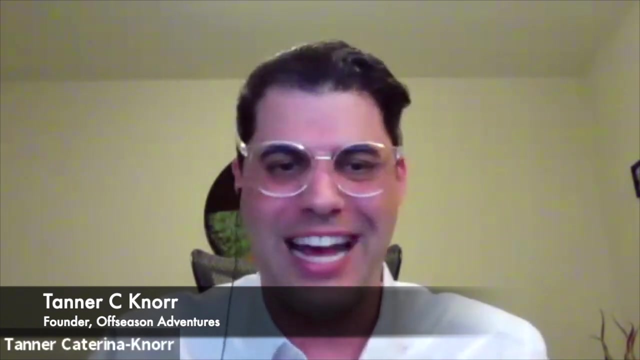 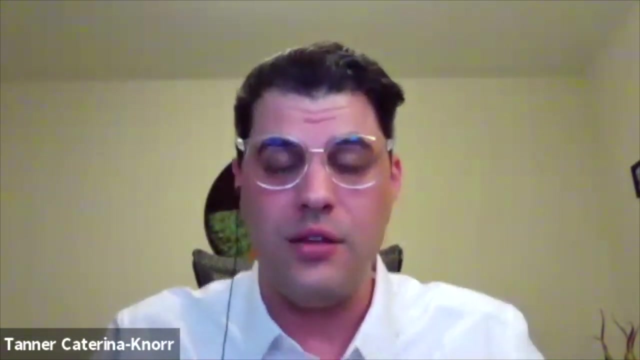 of other cars or other travelers in that space with you, so you really feel like it's all for the traveler. Over-tourism has several different aspects. There's a few ways to define it and several impacts that it brings to the destination. I like to think of it in terms of sustainability. so if we're thinking 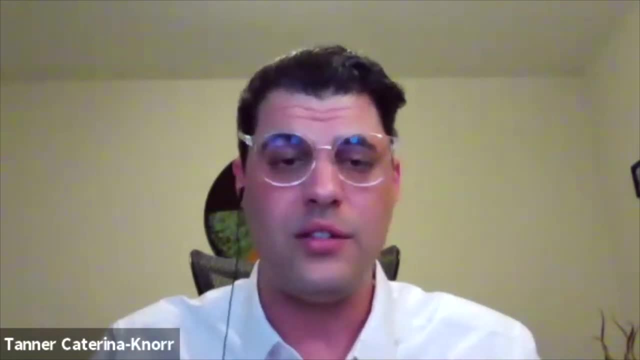 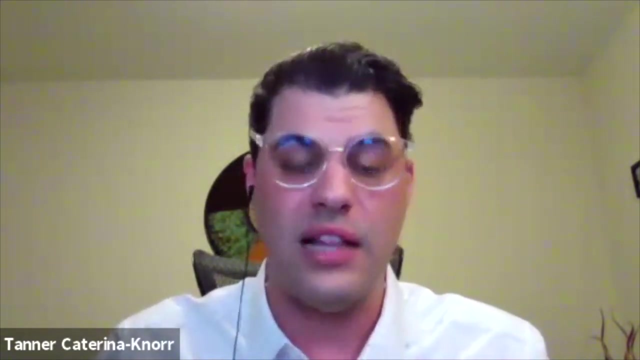 sustainability. we have those three primary pillars, so the social, the environmental and the economic. When we have a situation of over-tourism- while we might not be seeing that specifically right now during COVID, because of the lack of travel, there are places that have actually experienced tourism growth. 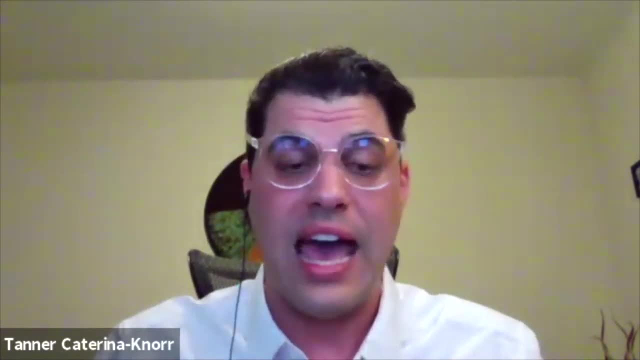 Here in the US, for example, a lot of our national parks have more travelers to them than they have in the past, and that still brings these challenges. My hope is that we can recover in a way that avoids over-tourism, and that we can recover in a way that avoids over-tourism and that we can 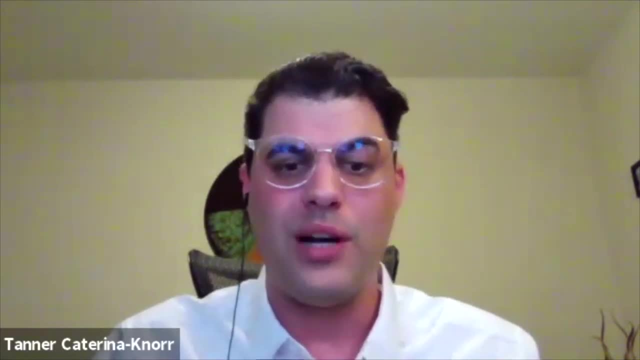 recover, especially now, without haftting that my experience from really seeing all of that tourism from happening in the first place. So again, if we're thinking about these three pillars we have the economic, social and environmental Over-tourism really affects all three of them. 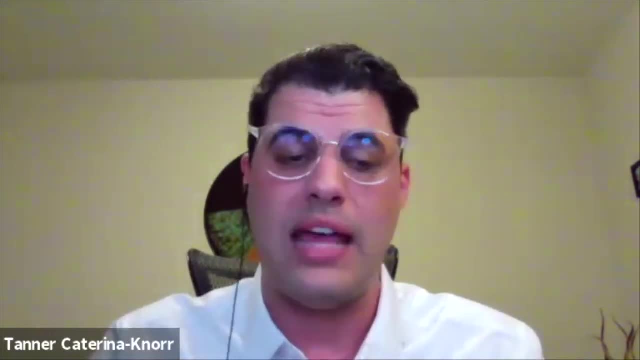 So if the destination is motivated primarily by economics and by that marketing of having more and more quantity of tourists coming to the destination, It will inevitably get to the point that there's two metabolism operates, having two left-hand, too many tourists for the destination to handle. 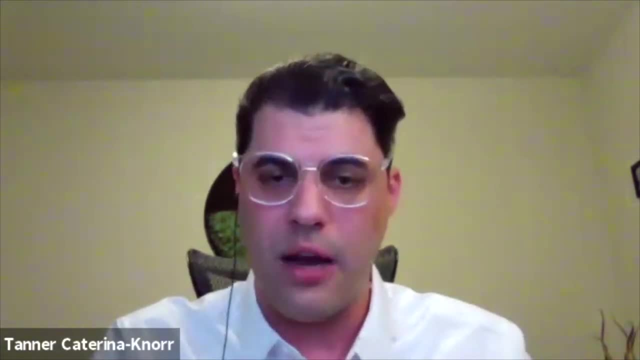 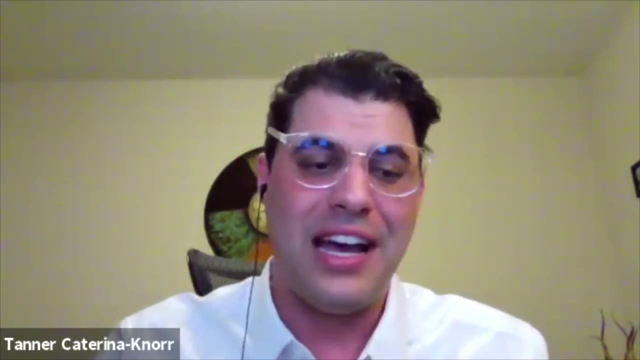 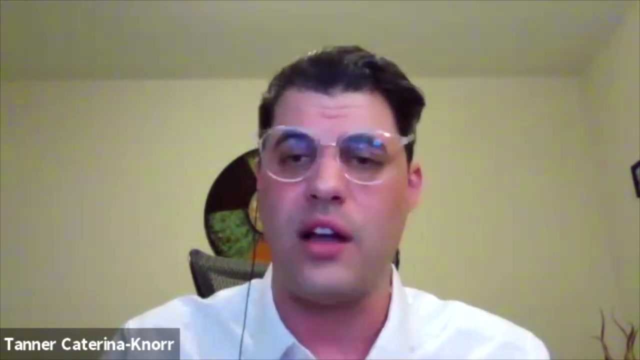 What this causes are primarily those social and those environmental impacts. So we have the environmental starting off with. we have the waste management issues, we have water management issues, sometimes in destinations, a lot of the common pool resources, So the national parks or the trails. 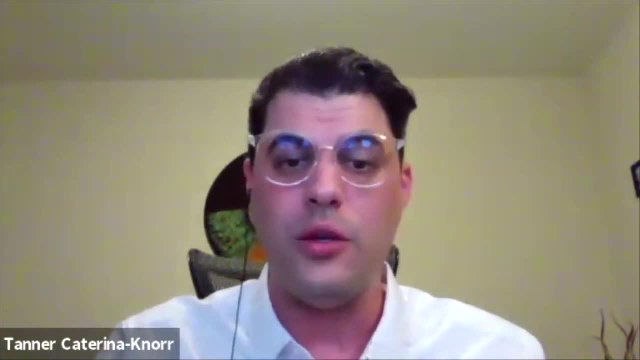 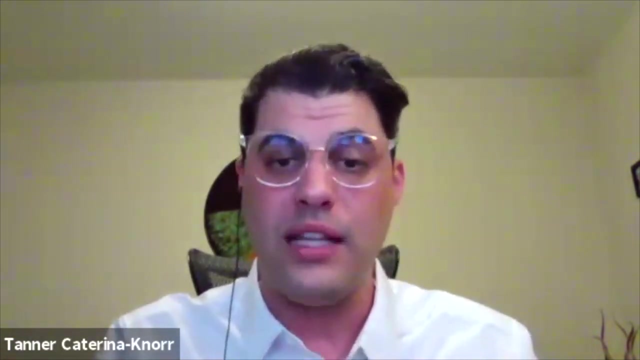 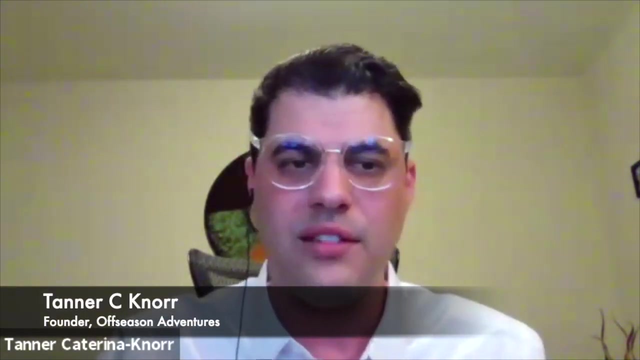 things that travelers and local people use together. sometimes there is a competition for those resources, and that's a situation that I think that all destinations would want to avoid, And then going along with those resources is how the people who live within the destination really handle compromising their stake in those resources. 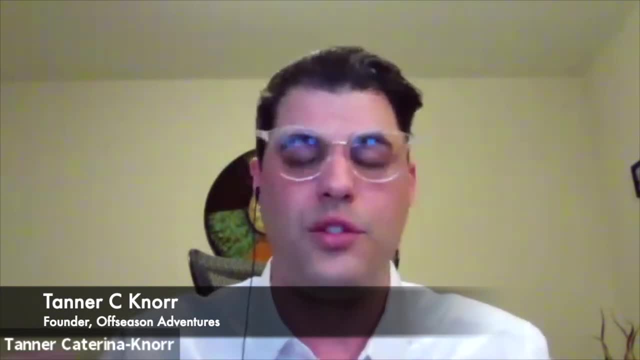 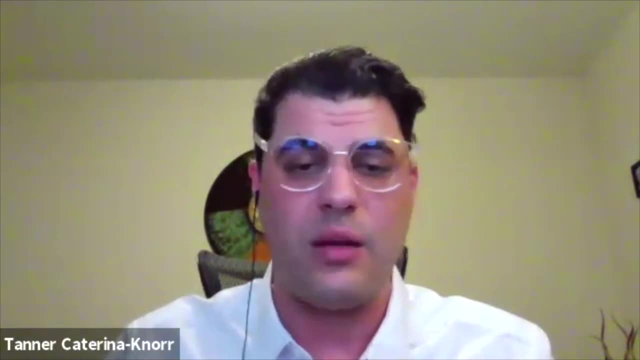 So if if there's a situation where there's too many tourists, let's say, for example, in South Africa, they had been dealing with a lot of water management issues over the last few years And what that's caused is kind of a clash between. 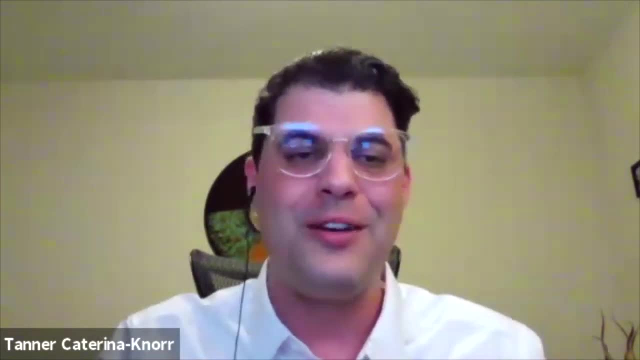 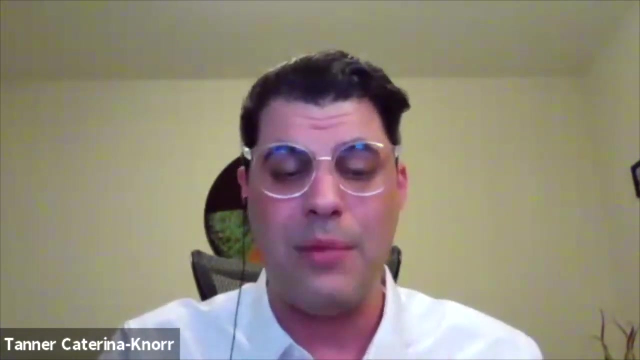 the locals who live there and also need water, versus the travelers that are coming to the destination. Traveling during the off season can help, you know, bring those things together. So the first in my mind is that environmental component. So traveling to a destination where there are fewer other travelers during that time. 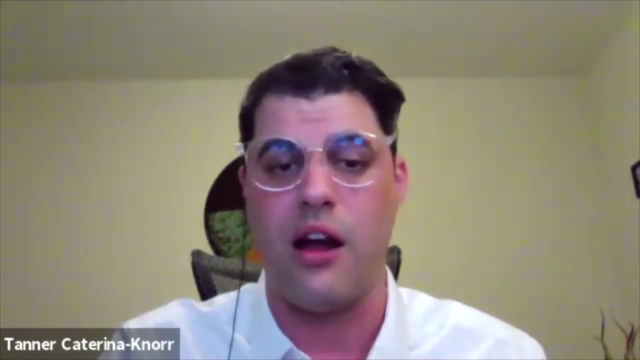 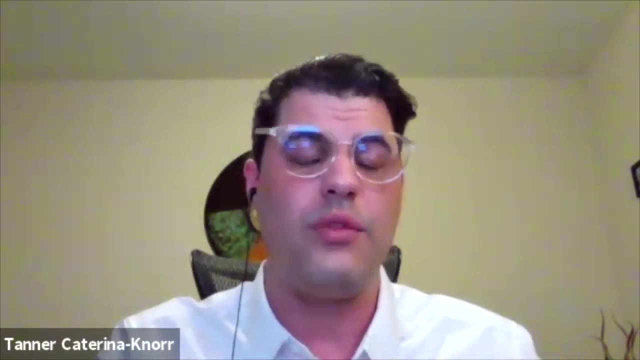 Really, the resources that are available within that space at a given time, then are are more per the amount of people that are there, So there's not as many issues perhaps, when, when, when, when, when, when. 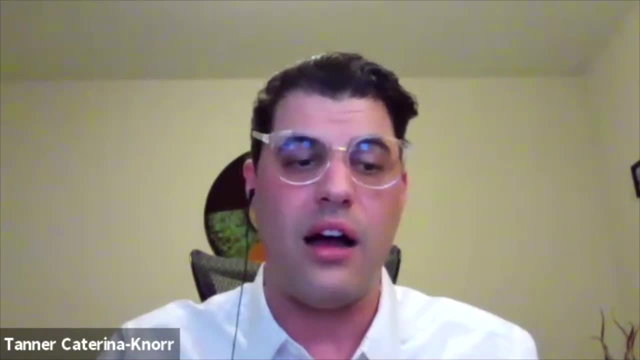 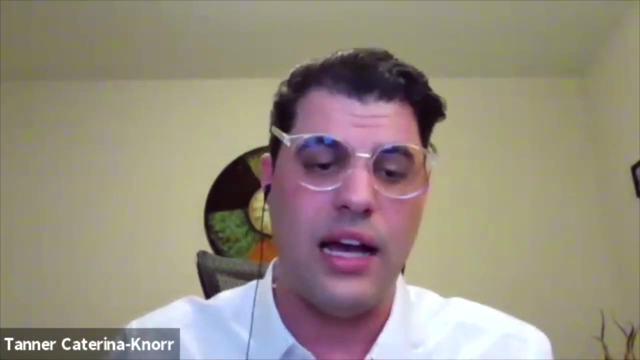 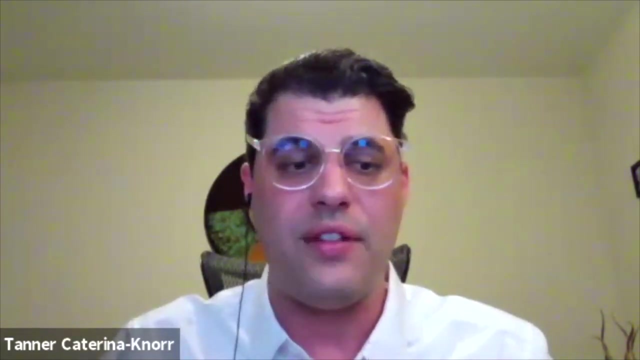 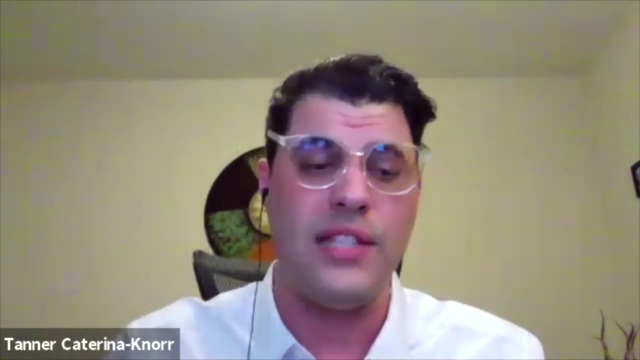 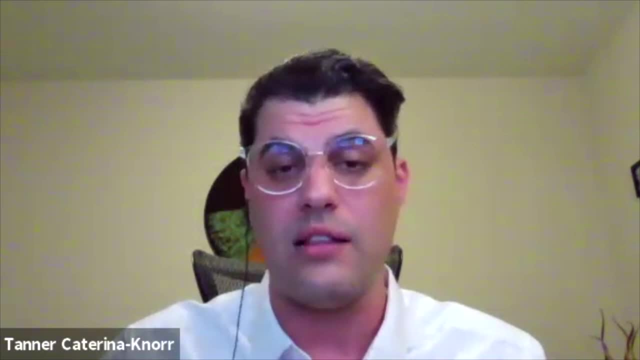 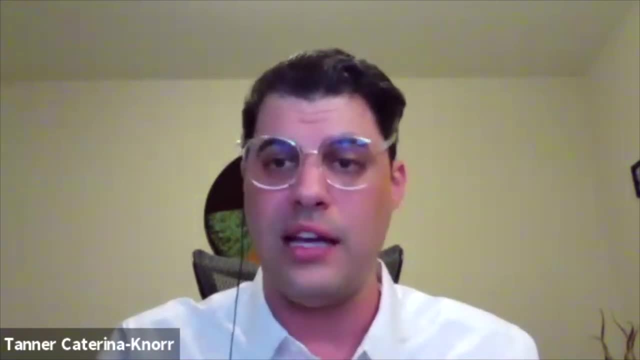 choosing to go maybe during a time of year where there are fewer tourists. but you also have the local policy makers, the government, the governance situation within the destination needs to perhaps sometimes move a little bit more away from the marketing component and more towards the management component of the destination. But then it also requires 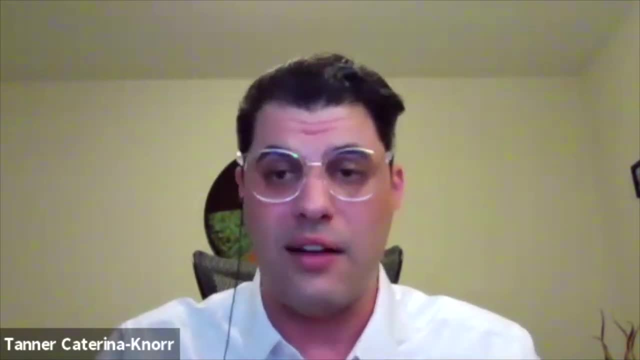 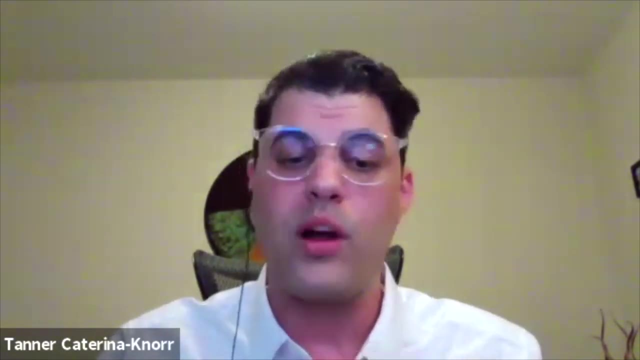 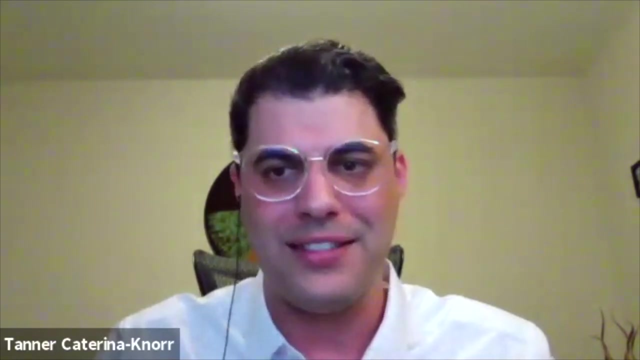 the tour operators that are sending travelers, like off-season adventures to Nepal, or Royal Mountain Travel, that's receiving tourists within the destination, working together to figure these things out, because it's something that one entity alone can't fix. So traveling during these four seasons can be responsible for supporting visitors. 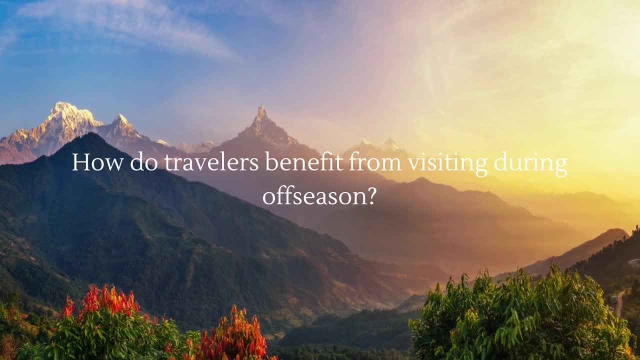 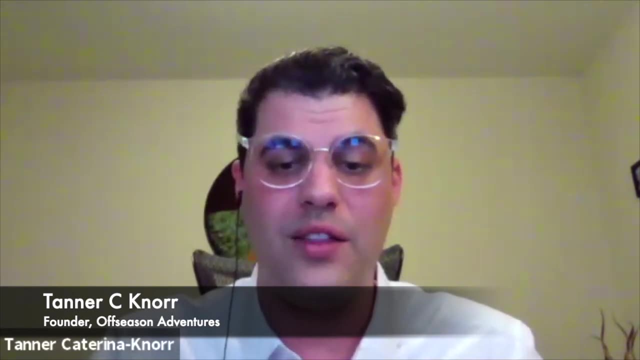 but rather in perhaps planning these NIH and NIH services to support that Flybackşı Province and the NLD她 or kitchen Moving from away. 그럼них los de года. So traveling during the completely off-season is fucking awesome. the off-season, in my opinion, is the best time to travel. This is where the travelers can have those. 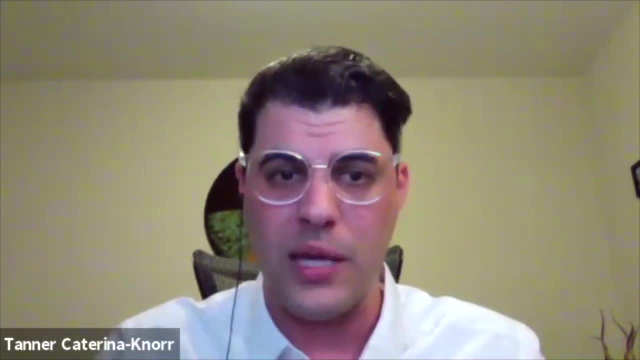 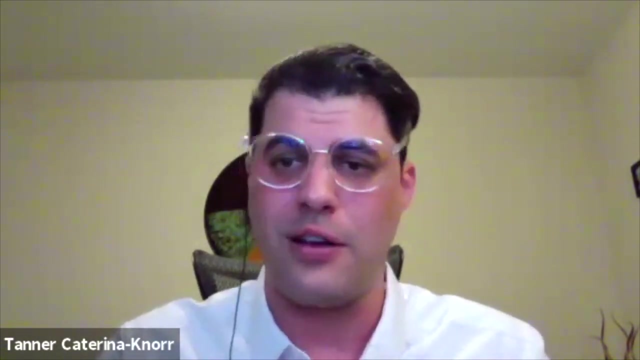 really personal connections with the local people. I've been to several destinations during the high season and it's just you don't have that intimate connection with the people because there's so many other travelers that are coming with you during that time. So if they're trying to show you how, 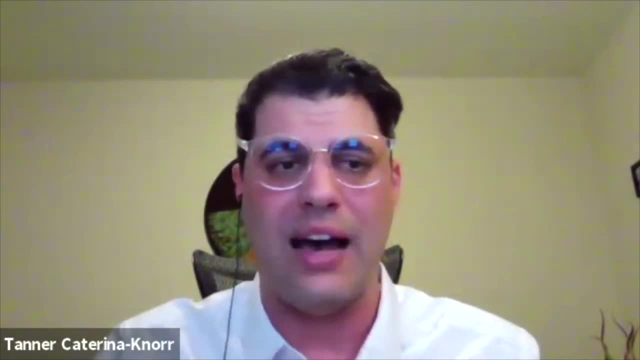 to make something or try and explain how they cook a certain type of dish. I mean, you can't have 20 people crowded around a kitchen at the same time, And so it makes it a bit difficult a lot of the times when you travel during the high season to have those really personal. connections with the people, But traveling during the off-season allows that to happen. The second favorite aspect of traveling during the off-season is that the entire landscape of the destination changes completely. So in Nepal, for example, when we're riding around Chitwan. 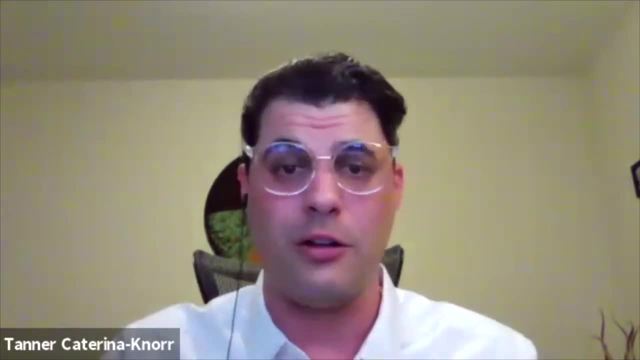 you have all of the rice fields that are completely in bloom and they're green and lush, and you see the clouds reflected in the rice, in the water, in the rice fields. There are rice pools there. It's just absolutely stunning. All of the mountains are lush and green. 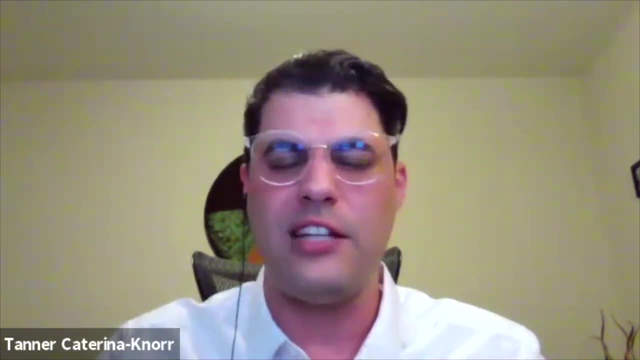 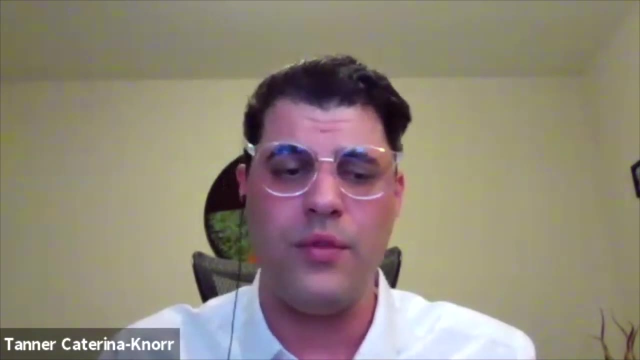 There's something to be said, too, for traveling during the off-season, in that the destination feels a bit more relaxed, Not only from the people and the tour guides, but also just the overall environment of the communities of Kathmandu Valley, even Traveling during the 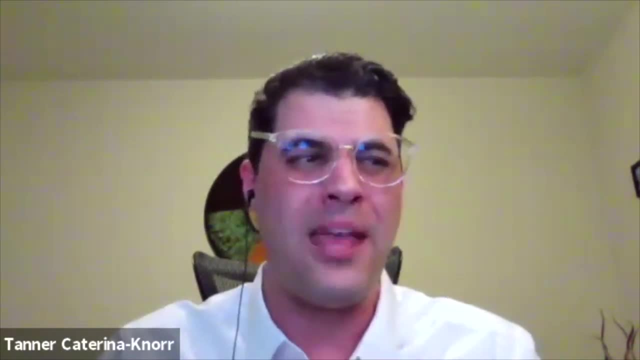 off-season is so much more relaxed. It's just so much more relaxed. It's just so much more relaxed. You don't feel like people are looking at you like, oh, there's another tourist, you know, just trying to buy some souvenirs. You know they really want to engage and have those. 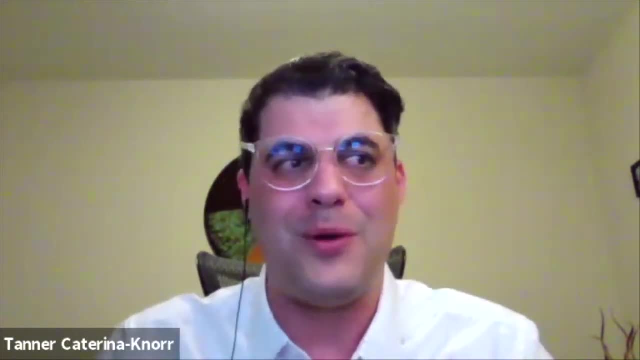 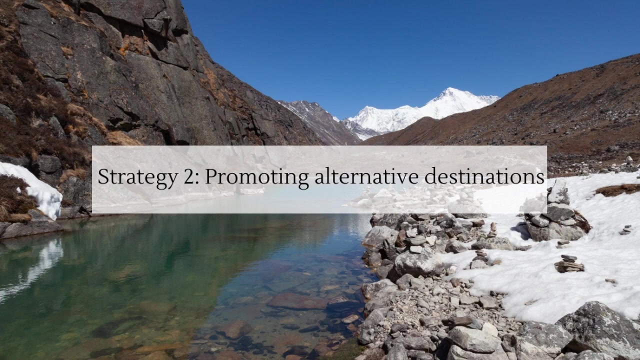 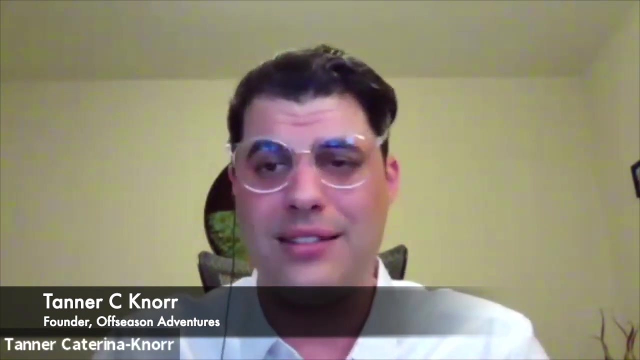 conversations, And for me, that's the most fun anyone could ever have, I think you know, when traveling abroad, having those really deep, intimate conversations with people. The thing about Nepal, though, is that there are so many beautiful treks right, And there's so many places to go in the country that people just haven't really heard about before. They don't know about, And so even if they are traveling during the high season and you know, let's say, they only have that amount of time off for work and they can't really avoid traveling. 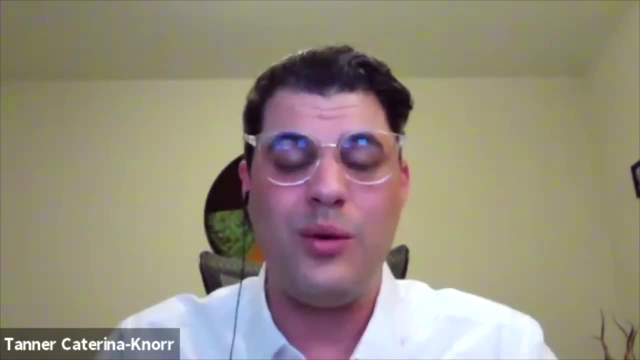 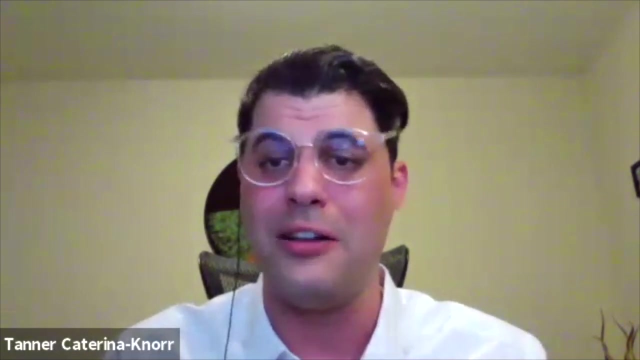 during another time of year. what we can do is work with you and work with Royal Mountain Travel and our other partners abroad to place our clients at places that are a little bit more untouched or unrecognized as places to travel, but still have really wonderful things to offer. So you get that sense of traveling during the off-season while still traveling during the high season. The homestays help to divert the traffic from highly popular destinations to the equally beautiful yet unexplored rural areas of Nepal. One of the examples could be Shirubari Village. 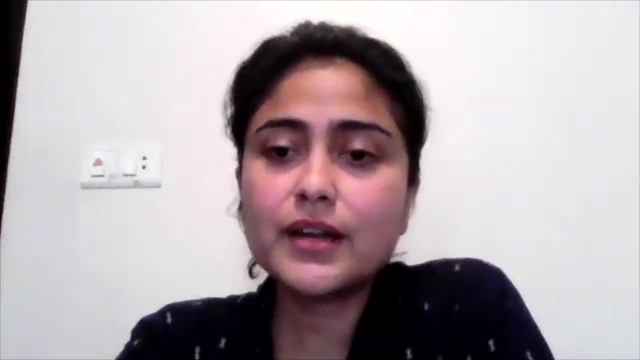 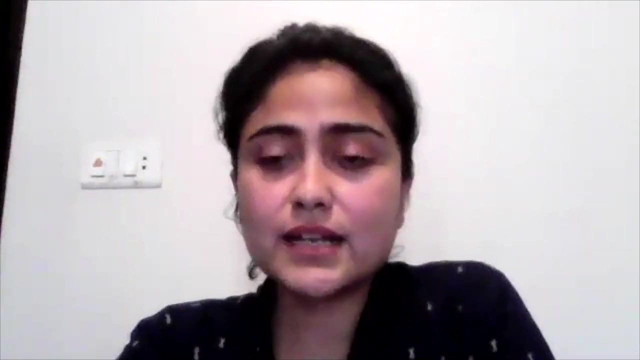 It is one of the earlier examples of community homestays in Nepal. So what Shirubari Village did was it just didn't promote the culture, tradition of the people who were living there, the gurum community, but it also helped Siamja itself to establish as a destination. 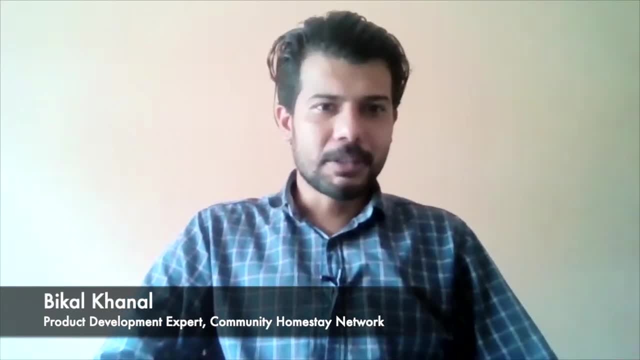 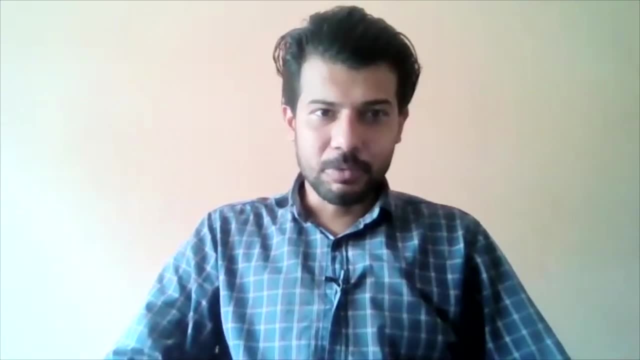 For traveling to Nepal. Annapurna region is one of the most popular places that people choose to trek, So this has been popular since 1980s, I would say, when travelers slowly started moving towards the mountain to cross it, And so the reason why there are such a lot of population here is because of the 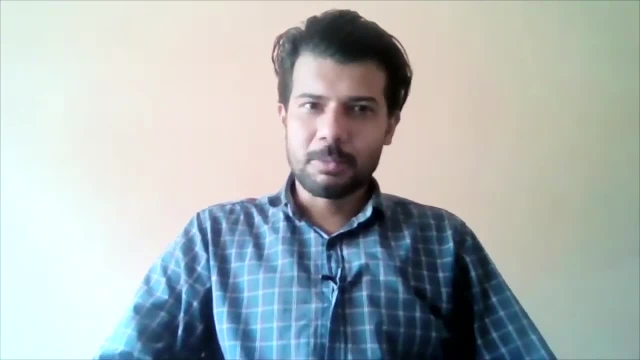 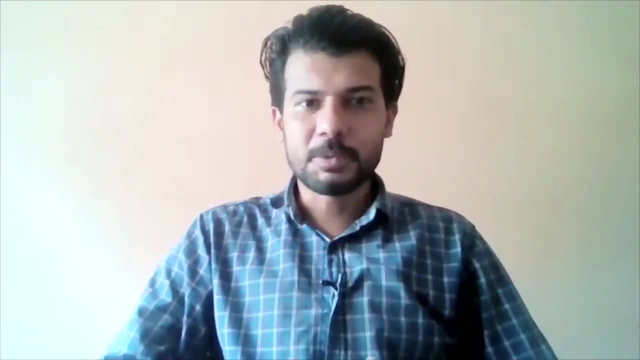 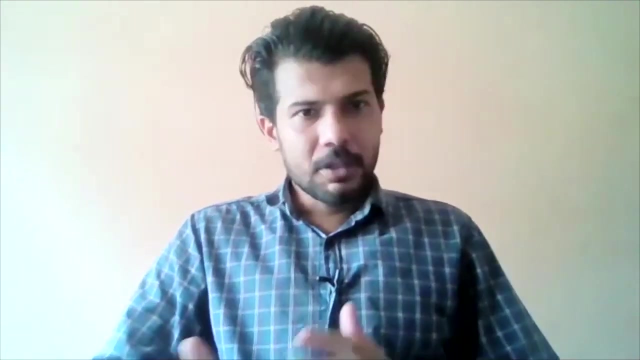 And then other various destinations were also developed, including Khori Pani, Khandruk, Mustang and many things. So Tathopani- it works as a hotspot, that the place is a transit where travelers come and accumulate. So usually what happens is when a transit destination is being hoarded by the people. 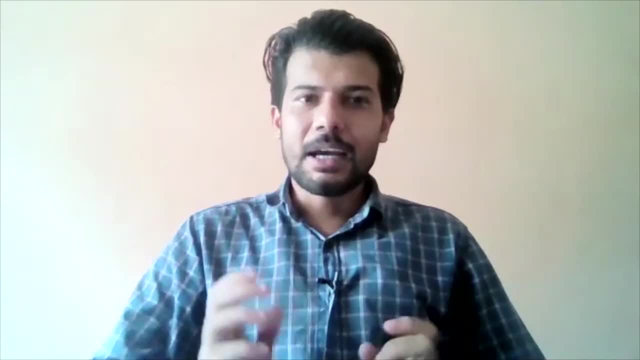 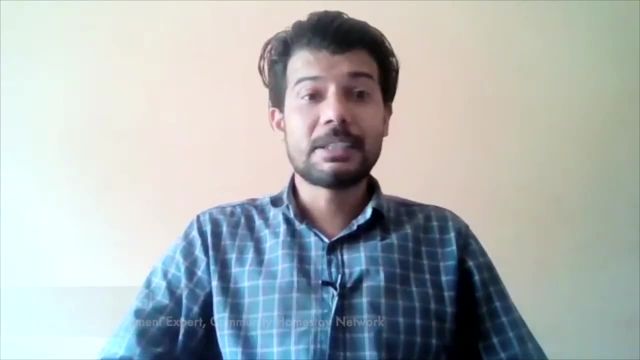 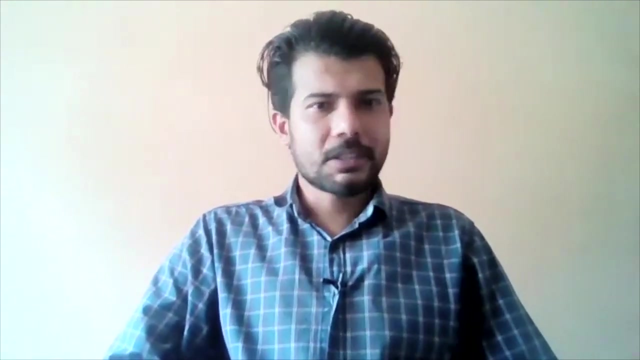 and few destinations like Tathopani and some of the others in Mustang and Manang. these places start to become a hotspot, where people have Put this place in their bucket list. So what happens is the place starts to get overcrowded. Right now, the situation is not so much escalated, I would say, because there are the tendency. 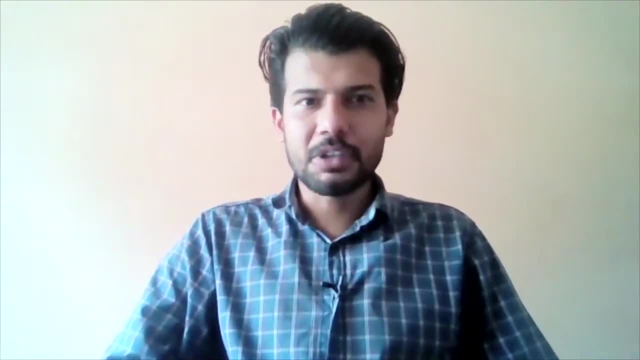 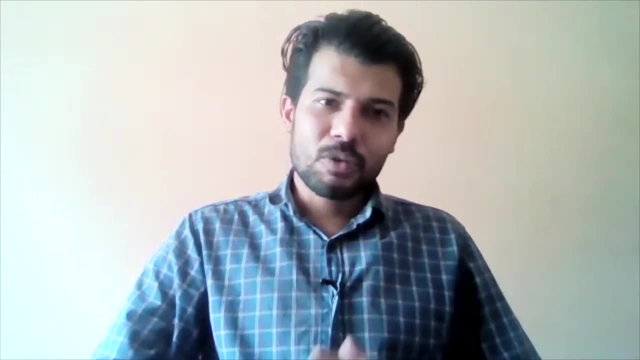 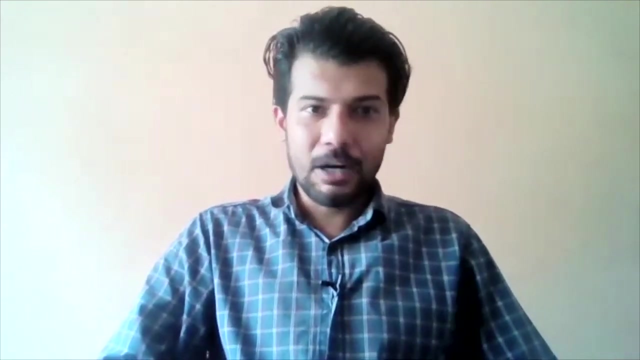 of the foreign travelers and international travelers doing the trekking most of the time, But as gradually the local tourism also is starting and as local travelers are also starting to follow this trend of trekking and going to the mountains, now we assume that a problem. 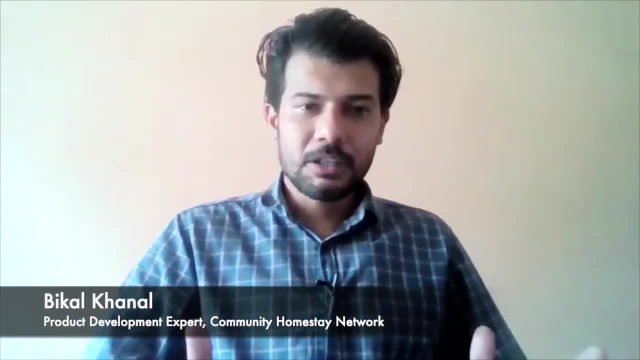 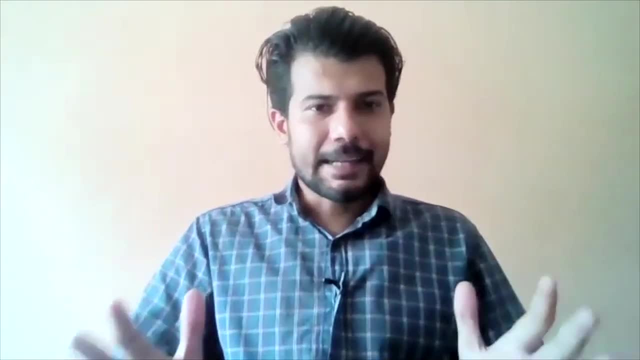 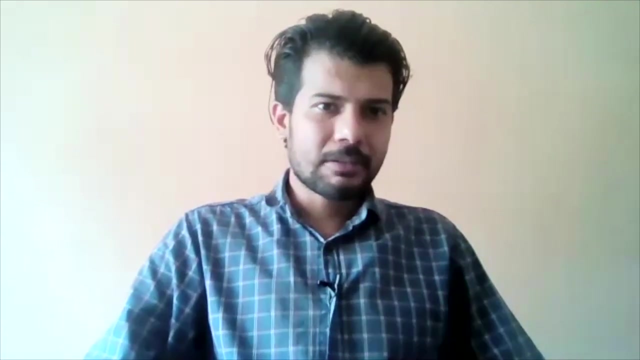 May escalate because Tathopani, if you see geographically the place, is a very limited town. I would say that has a capacity to that has a capacity to hold a number of peoples, but it has its expansion limits. It was somewhere around five, six years ago when I first visited Tathopani and recently 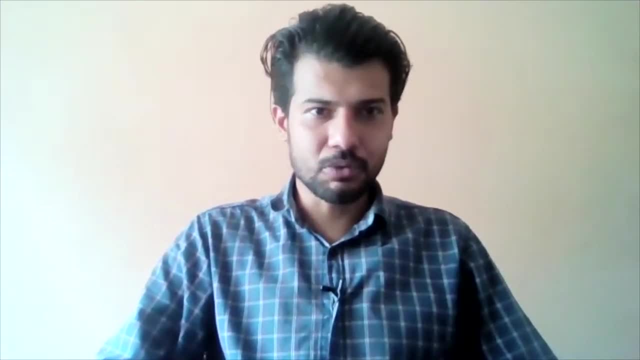 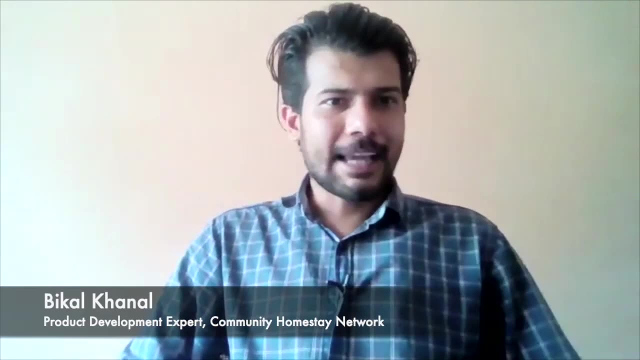 a few months ago. So there has been a drastic change in the city to accommodate this growing demand. So we can clearly see that the demand is growing. So to tackle this problem of growing demand in the region, we were always looking for an alternative. 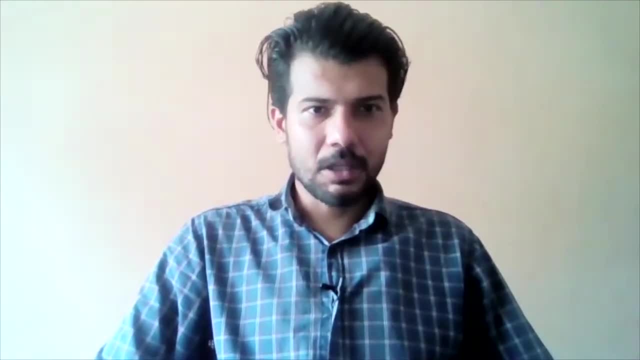 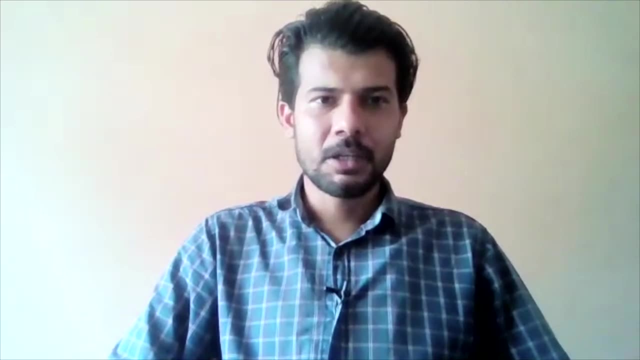 Then, with the help of a colleague who was a local of the region, we found out a village that was just 45 minutes walk from Tathopani, just across the Marsangi River. The village was Nacang, so we initiated to create a community homestay project there. 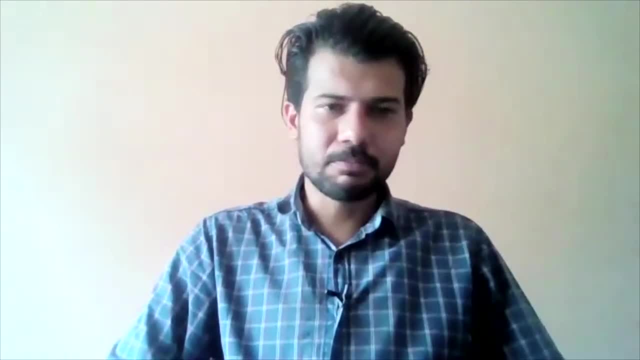 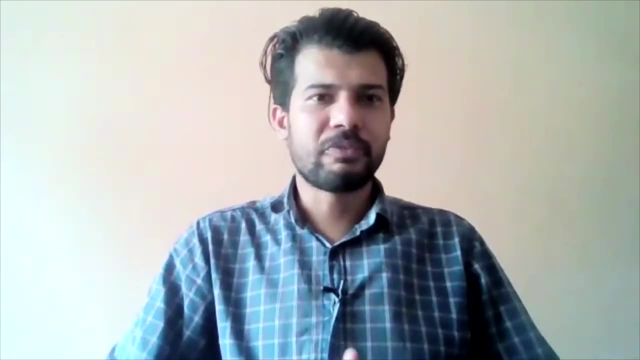 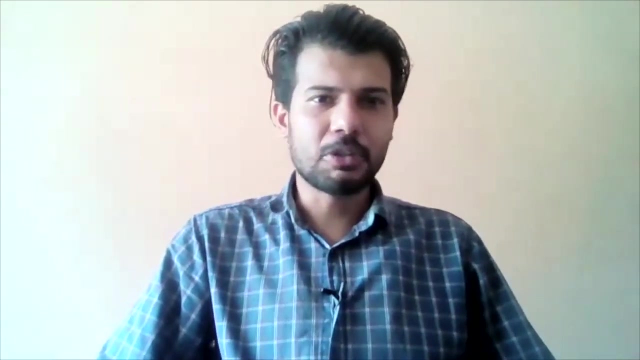 that would give travelers an opportunity to live in a pristine and peaceful place, with mingling with locals and trying to get the feel of the real Nepal. So what is the significance? The question has always been like: what is the significance of Nacang community homestay? 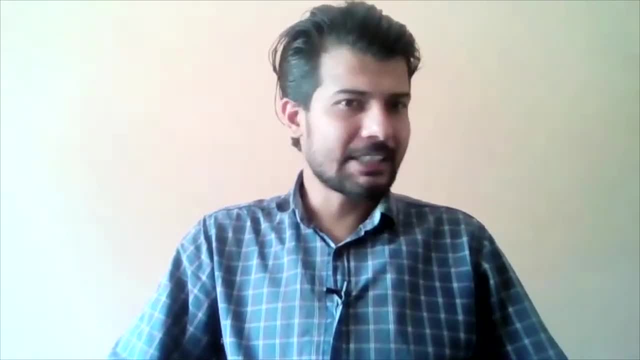 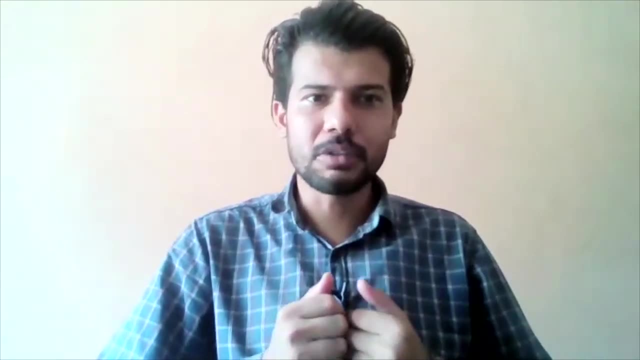 to tackle this problem over tourism. So the first thing is Nacang community homestay can act as an alternative destination to people who are actually looking for a little peaceful environment And people who want to live in a peaceful environment And people who want to live in a peaceful environment. 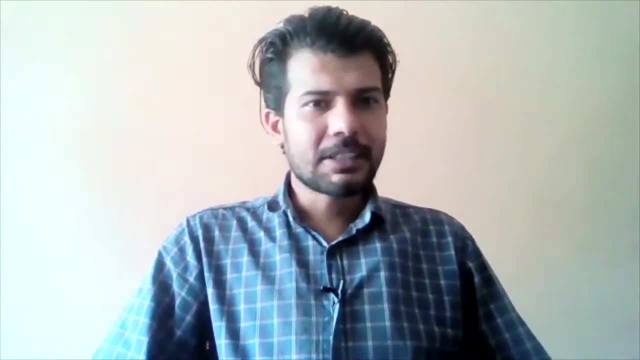 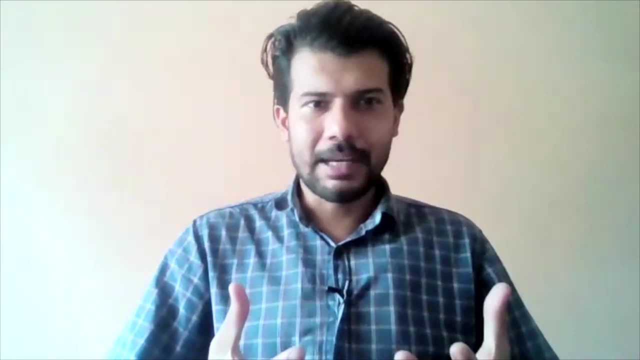 And people who want to live in a peaceful environment. So the first thing is that we have a good, in-depth conversation and experience with the locals. Also, Nacang community homestay can also be an example, as it will eventually, we presume. 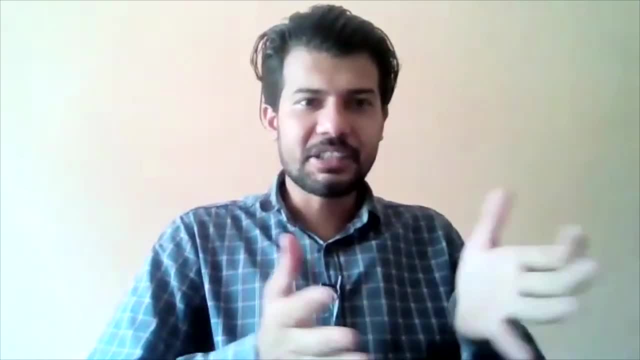 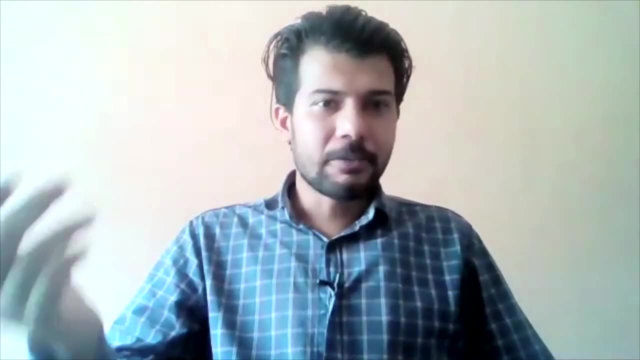 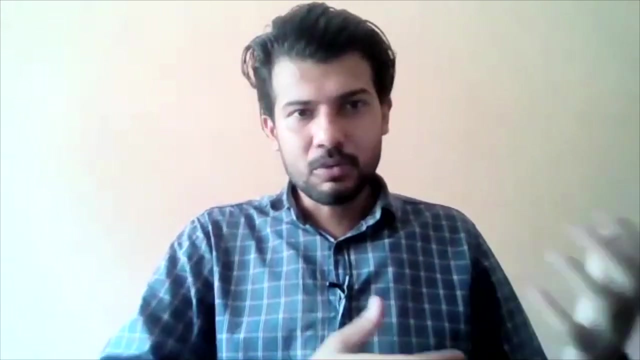 it will stand out as a model that will help redirect this flow of visitors from a concentrated place to the overall area, so that other nearby villages also start to get motivated. They see the prospects of tourism and they also eventually start creating their own tourism businesses. that will create a lot of alternative options within the region and also. 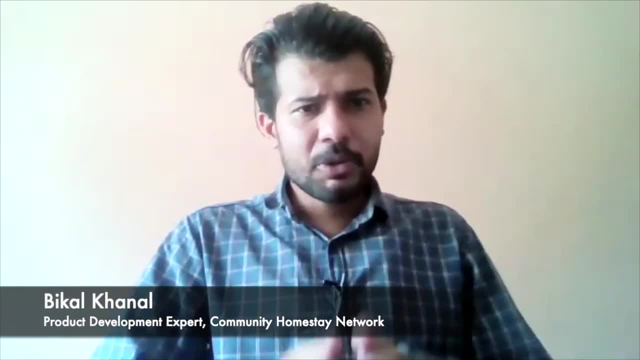 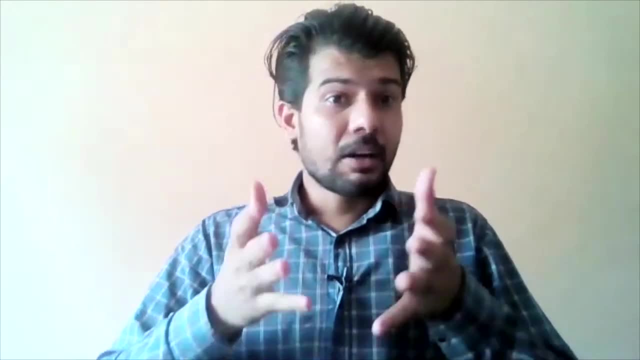 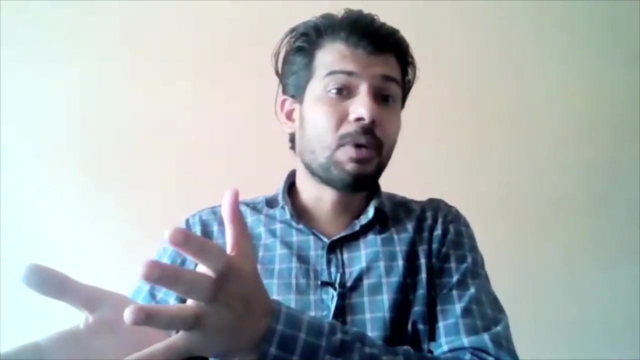 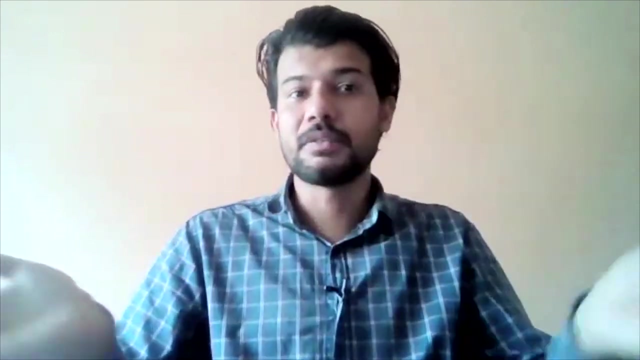 when we are, we are also talking about the community-based tourism and local tourism. this alternative destination- directly tackling the problem over tourism- will obviously help in a lot of a lot of aspects. as there are less number of tourists in one concentrated location, the resources doesn't get too much exploited as they would be because of all all those birds of. 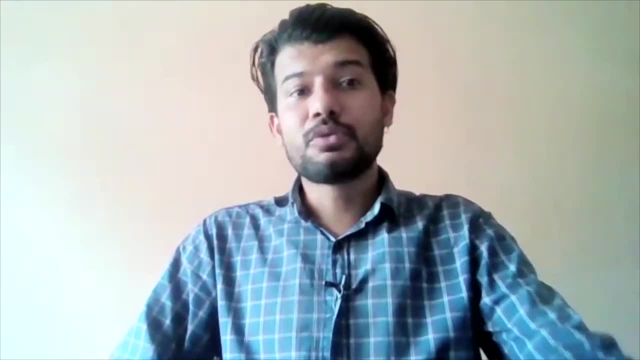 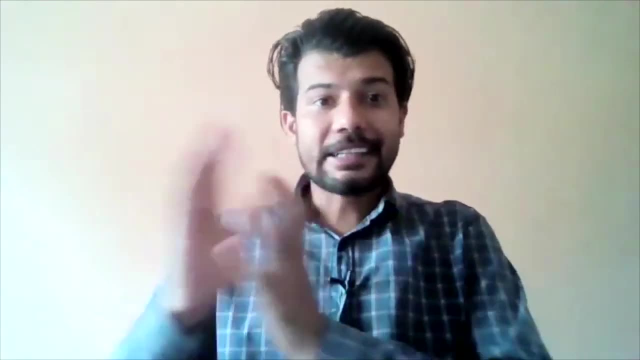 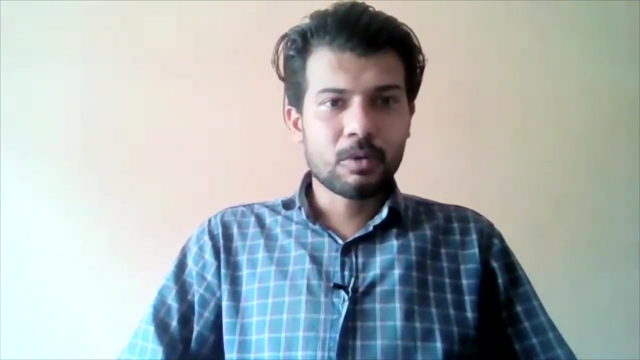 people and also it would add a value to the overall region as well. projects like this has been initiated, so the benefits will go directly to the locals, the visitors. they can also mingle and participate in the daily activities local, so this will give a overall summation experience. 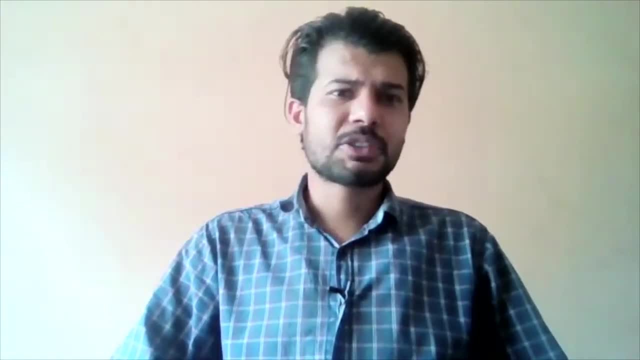 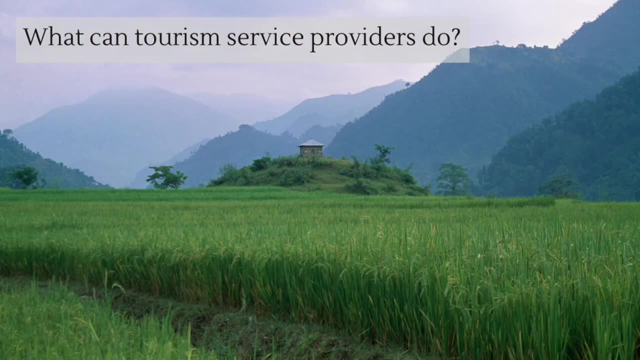 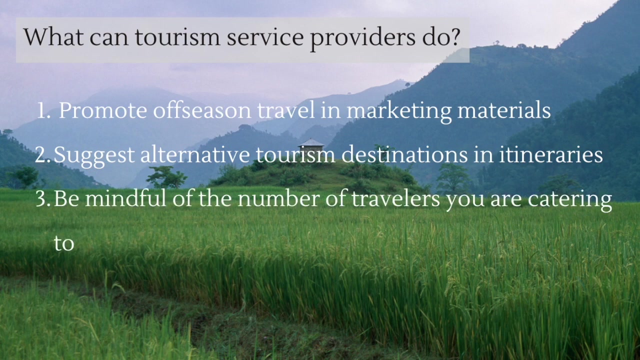 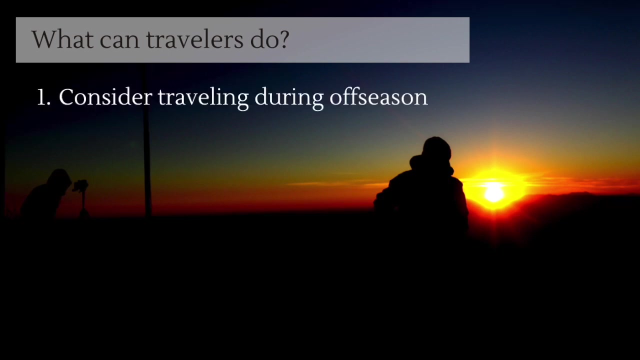 a different experience of nepal to the traveler who had been stopping by tea houses and walking treacherously all the way across the trails with the local tourism funders to get the benefits they need from the tourism and local tourism helping bring the local tourism to the people of the region. you know it's, it's, it's a never.